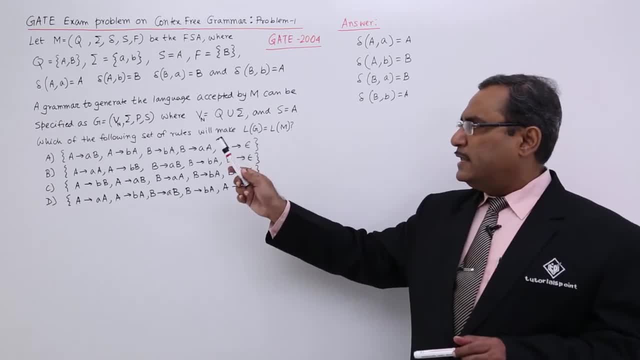 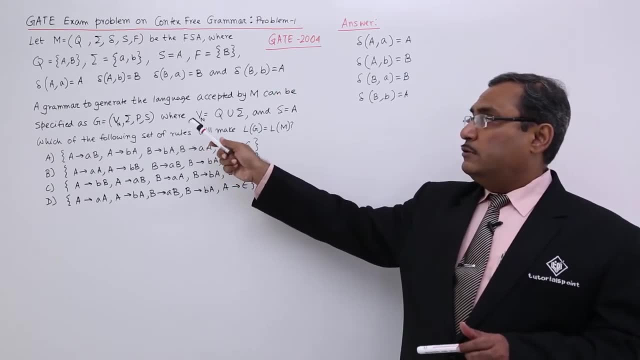 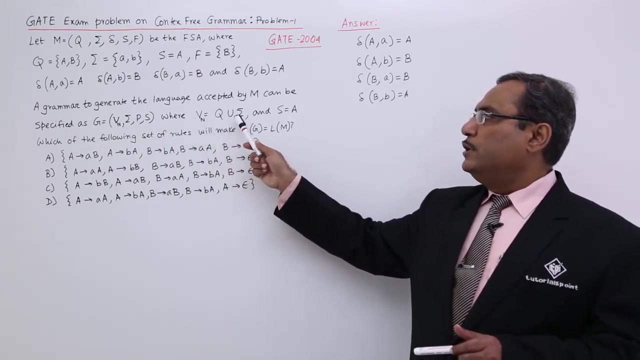 accepted by M can be specified as: G is equal to VN sigma PS. So from that finite state automaton they are trying to get one equivalent grammar. So here it is VN sigma PS and VN is equal to Q. So union sigma, that is a set of states, union set of input alphabets, And S is equal to. 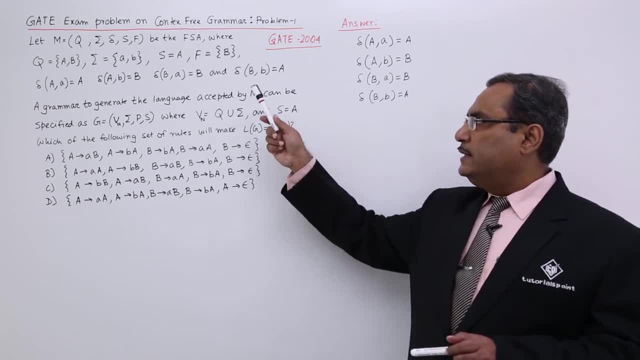 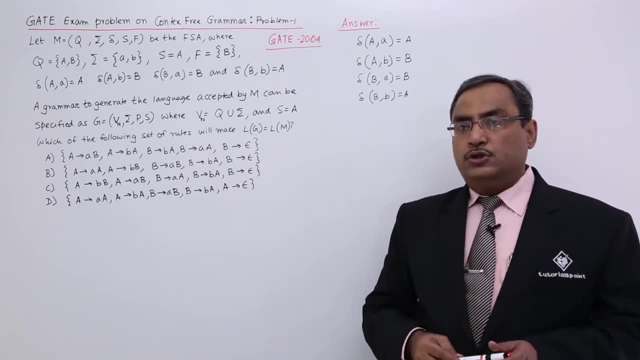 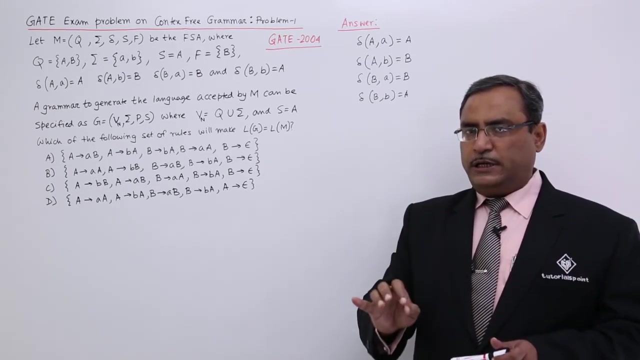 A- So that is a start symbol- will be A. That is the initial state And which of the following set of rules will make: L of G is equal to L of M, So finite state, automaton has been given and you shall have to find out the respective equivalent context, free grammar. So here: 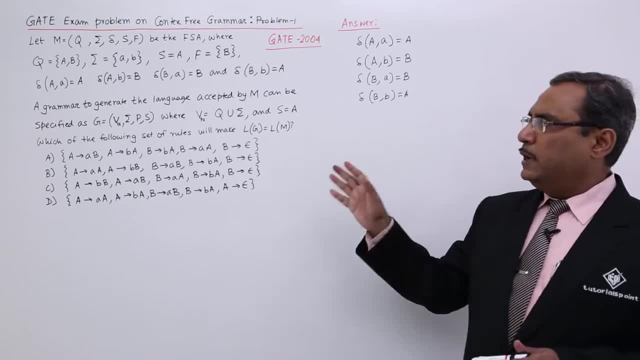 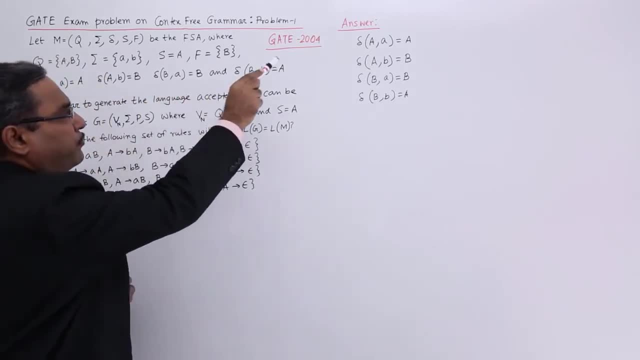 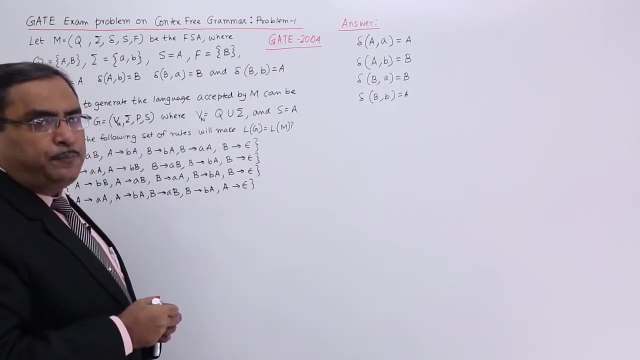 lies the problem. So how to solve it? So it is a typical type of problem. This sort of problems might be coming See. So here I have written this: four transitions I have written from the question paper. Now, against each and every transition, I shall be writing the respective: 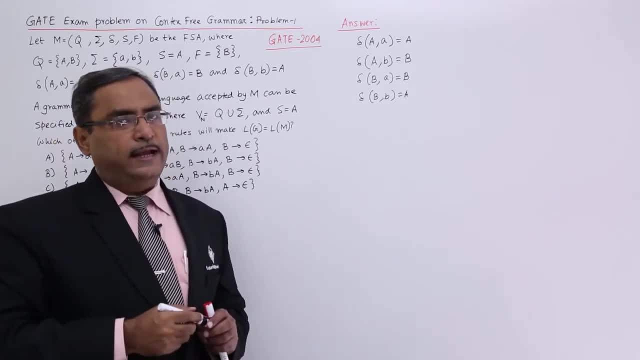 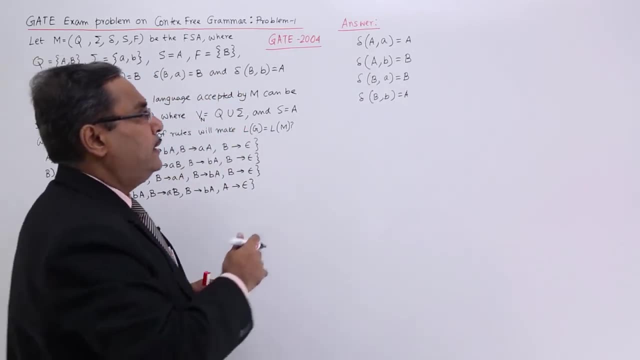 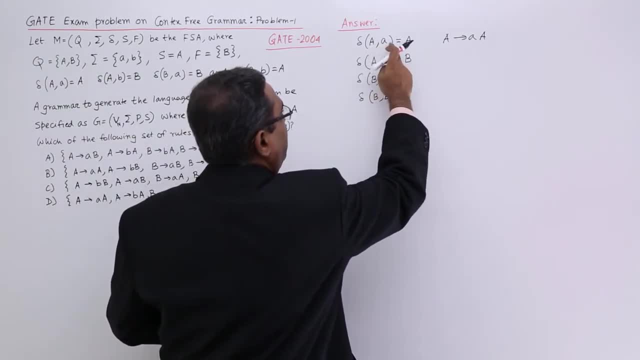 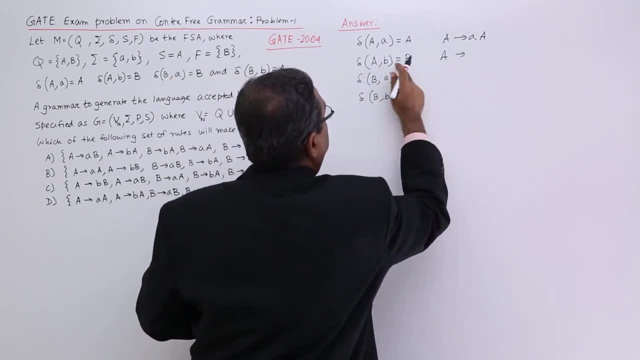 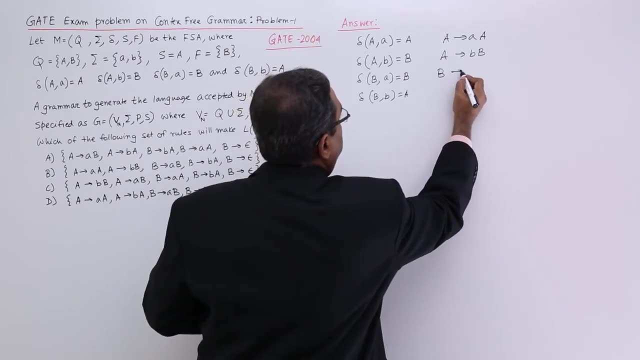 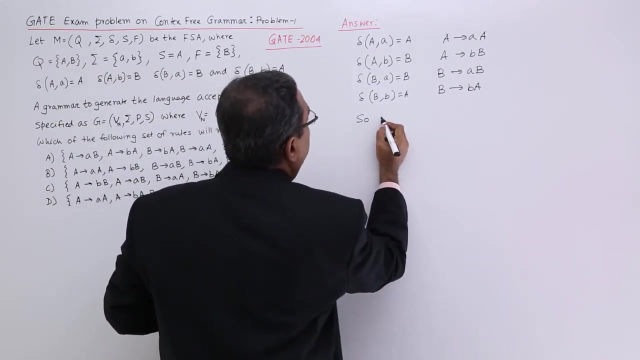 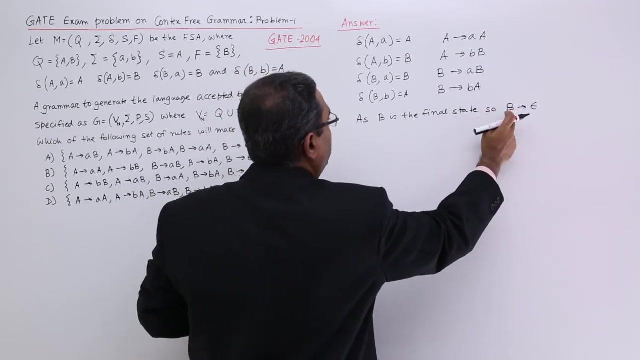 from this one. where should I go? I should have this: produces bb, A produces bb, So from here, B produces ab. From here B produces ba Now, which is the final state b, So b. B produces BA Now, which is the final state B, So B as B is the final state, so B produces.